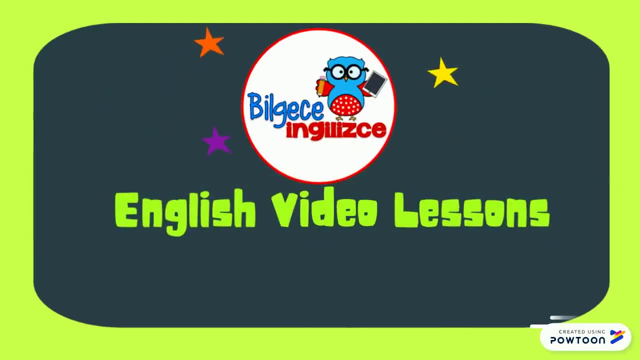 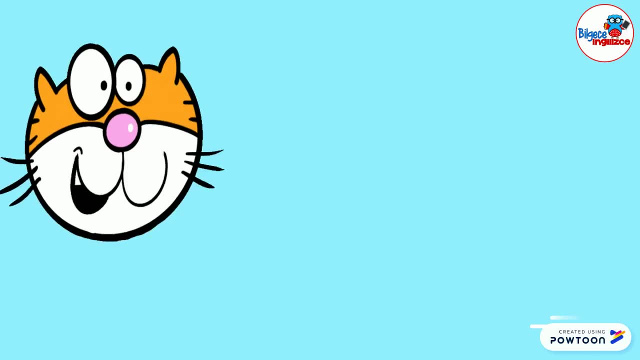 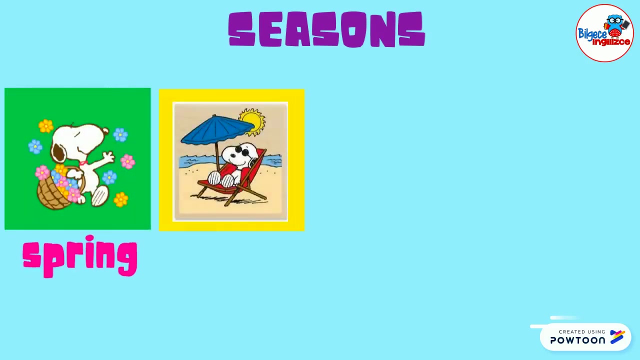 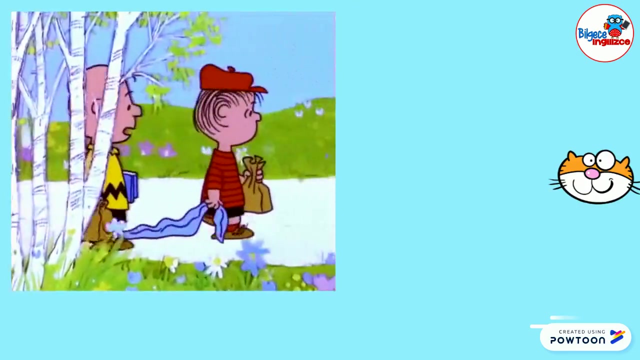 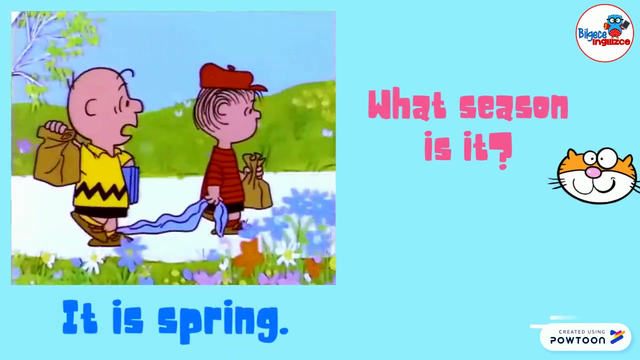 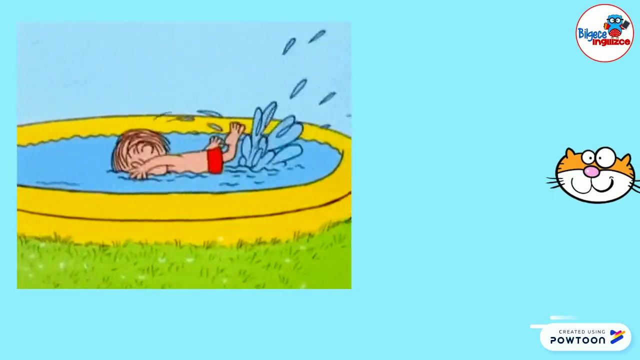 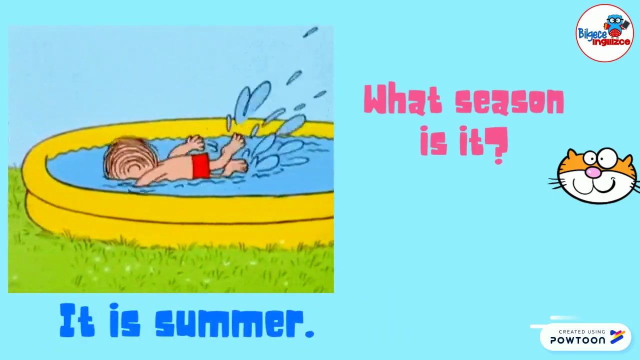 Hey everyone, Let's learn seasons and weather. Here we go Seasons: Spring, summer, autumn, fall, winter. What season is it? It is spring. Spring, It is spring. What season is it? It is summer, It is summer, Yes, summer. 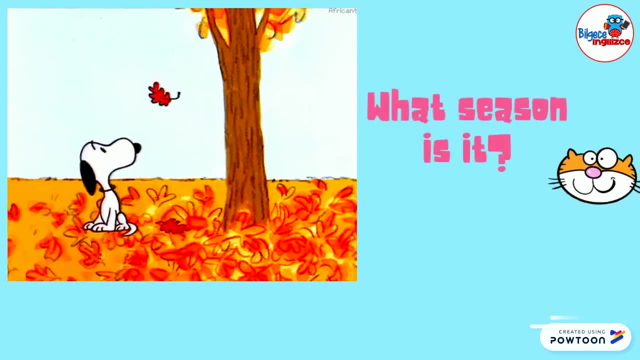 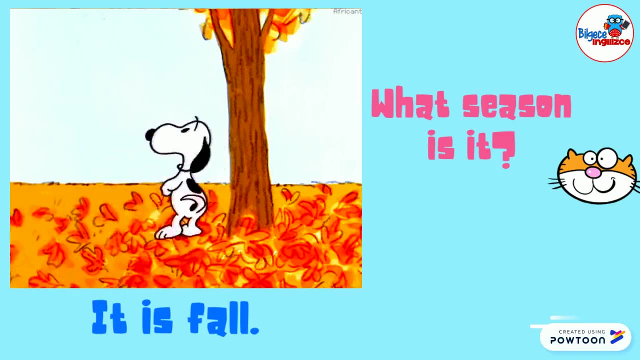 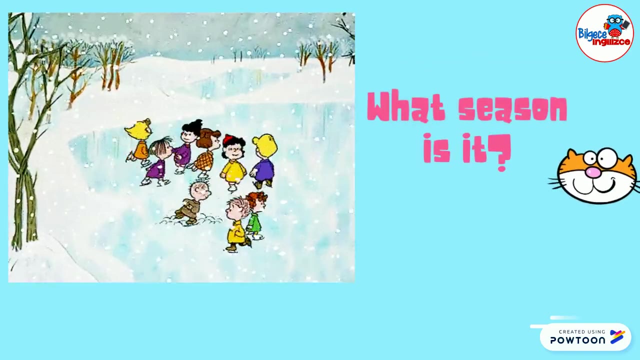 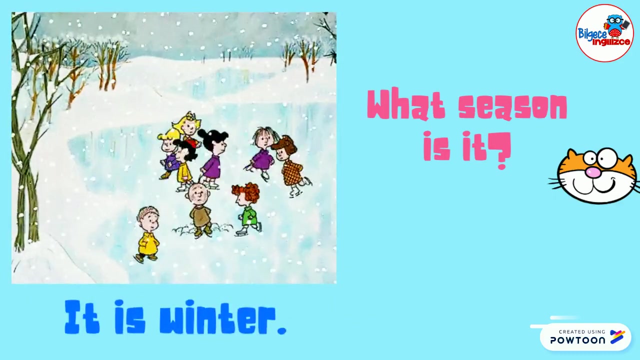 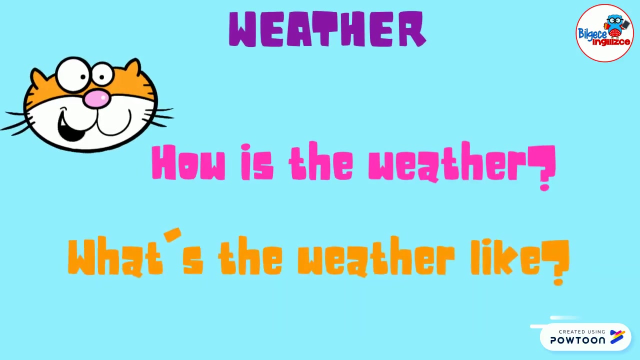 What season is it? It is fall, It is fall. What season is it? It is winter. It is winter. Yes, winter Weather. How is the weather? What's the weather like? How is the weather, What's the weather like. 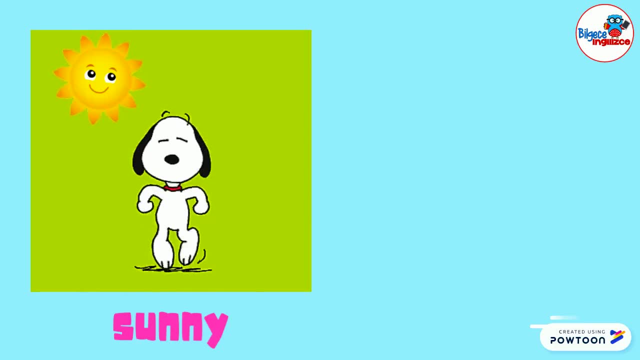 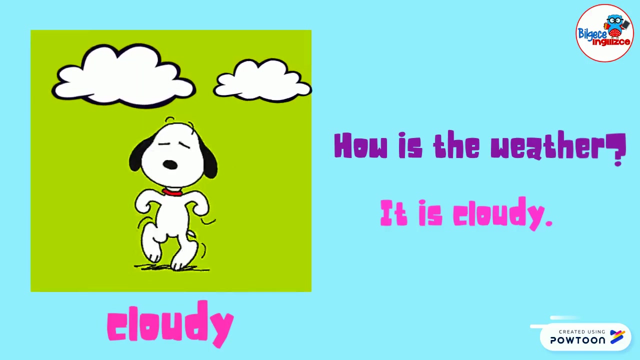 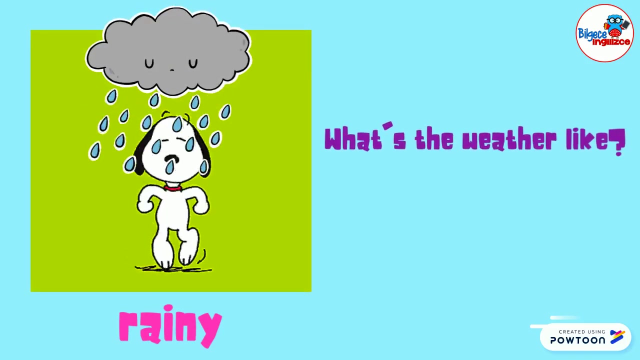 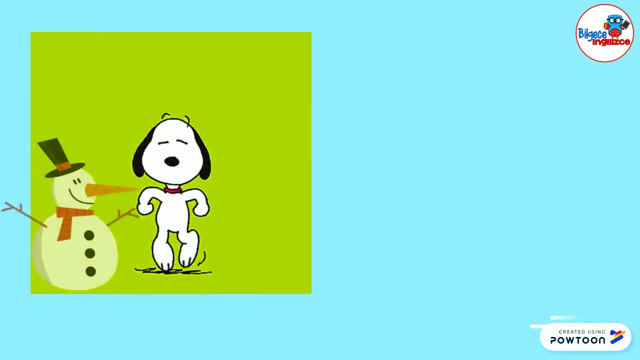 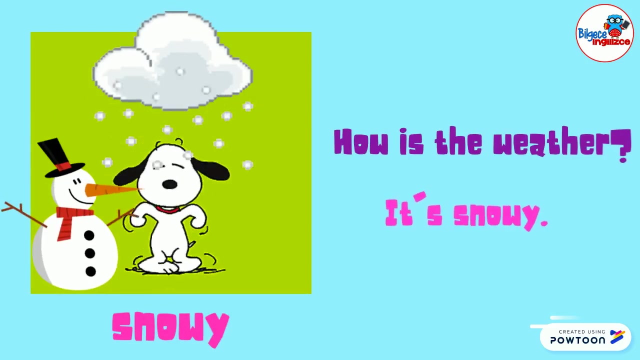 Sunny. How is the weather? It is sunny. It is sunny. Cloudy. How is the weather? It is cloudy. It is cloudy선이. Yes, it is cloudy. It's rainy. What's the weather like? It's rainy. It's snowy. How is the weather? It's snowy.